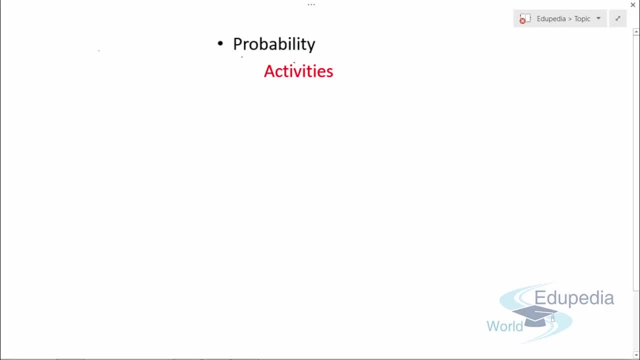 Hi there, welcome to edupediaworldcom. You're watching the videos on probability, So in this video we'll discuss some of the activities related to probability, how we can apply our experimental approach to prove the probability concept. So we'll be discussing some of the 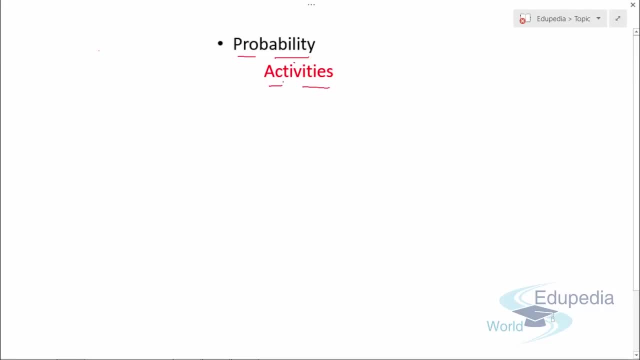 activities which you can find useful and which will also help you in solving the exam style questions, right? So let's get started with the first activity, which is activity number one. Okay, activity says that take any coin, toss it 10 times and note down the number of times a head. 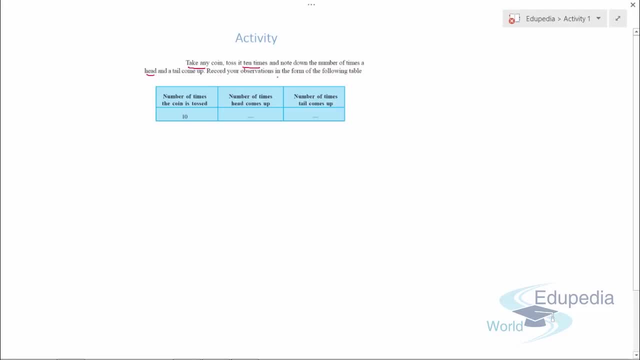 and tail comes up right, And then you record your observations in the form of following table right. So let's say these are the number of times the coin is tossed, let's say 10 times. And then we need to observe, let's say number of times head comes up, let's say it comes out to be 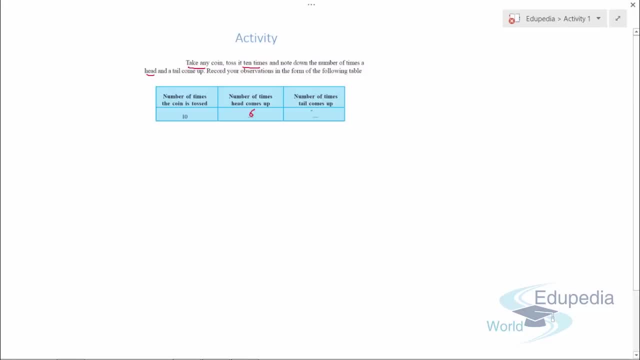 six times right, And number of times the tail comes out. let's say it comes out to be four times Now. so you always have to remember that the number of times the head comes up plus the number of, let's say, number of times head comes up plus number of times tail comes up, should always be. 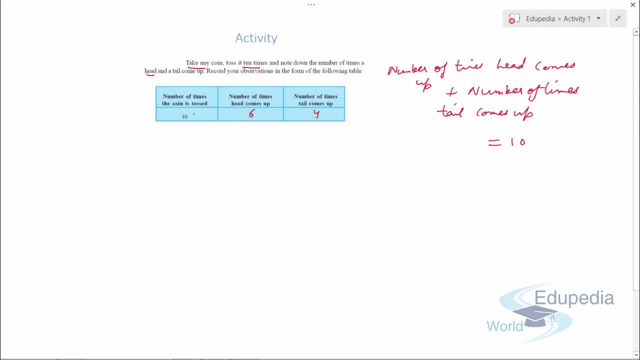 equals to 10 means these individual events should never cross the total number of events. So this is a very important point you have to always remember in your mind. right Now, what we need to do is we need to remember that the number of times the head comes up plus the number of times 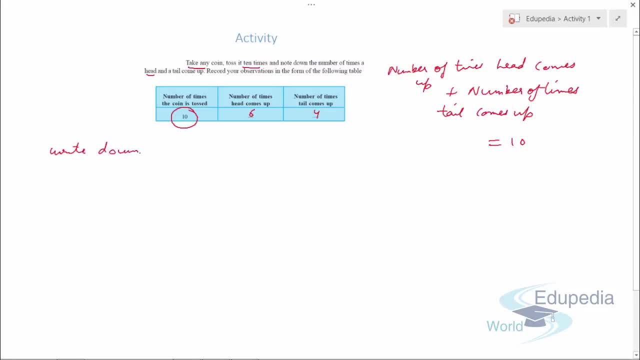 the coin is tossed, right. So this is the values we need to write down. We need to. then. what we need to do is we need to write down values of the following fractions, right, Let's say. first one is: you can write number of times a head comes up upon total number of times the coin is tossed. 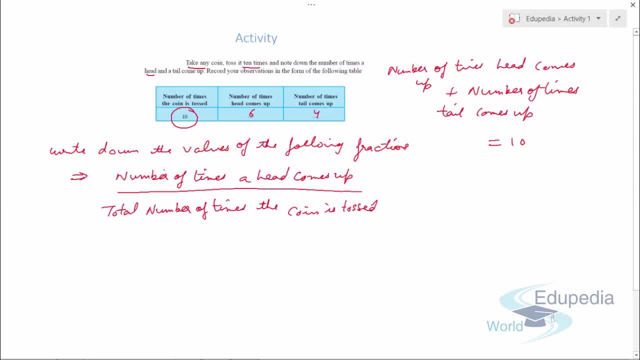 right. So this is the values. We have to note it down. Let's say the number of times the head comes up is 6 upon the total number of times the coin is tossed. This is 10.. So value comes out to be 0.6, right. So next value we need. 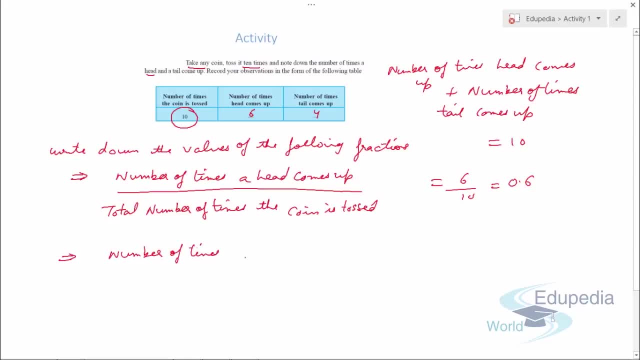 to note down is number of times times a tail comes up upon total number of times the coin is tossed. Let's say it comes out to be 4 by 10.. So this comes out to be 0.4.. So these are the values we have obtained when the number of times 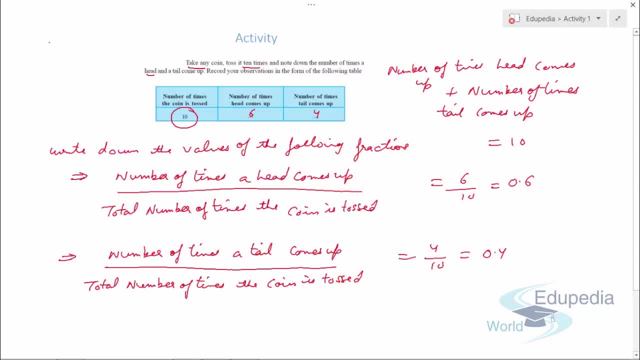 a coin is tossed is 10.. Now, next point is: let's say, toss the coin now 20 times, right? So, and in the same way, you need to record your observation as above, Again, you need to find these values. 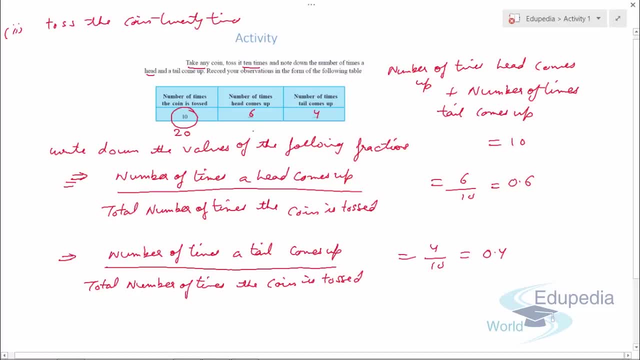 right. Let's say, if you toss the coin 20 times and let's say the head comes out to be 13 times and the tail comes out to be 7 times, right? Then again you need to find the fractions or values like this. then you again need to repeat the observation for the higher. 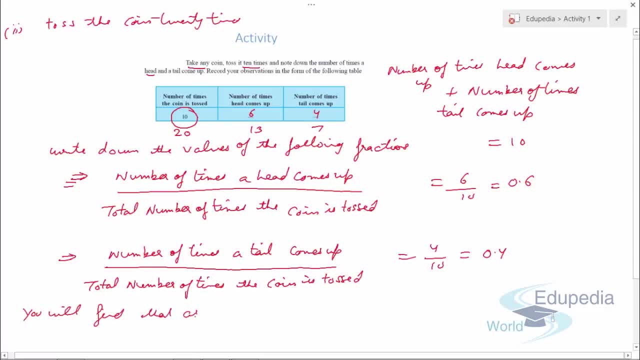 values. And then you will find that as the number, as the number of tosses gets larger, right. So as the number of tosses get larger, the value of fraction will approach to 0.5, or we can say it will come closer to 0.5.. Why? 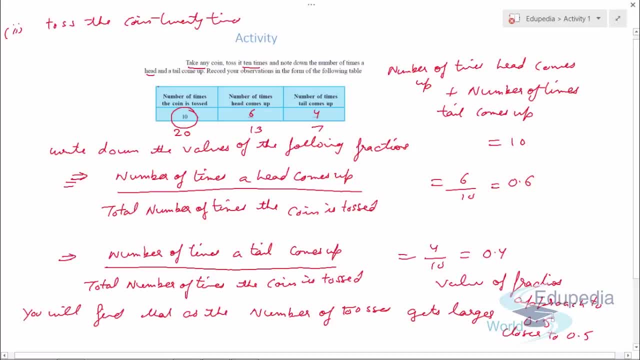 Because, as we have already discussed, when we are applying experimental approach- let's say we tossed a coin once only- So the probability of coming head and tail is 50-50, right. So whenever we apply experimental approach, we have to apply unbiasing, we have to be very neutral, right? So whenever we 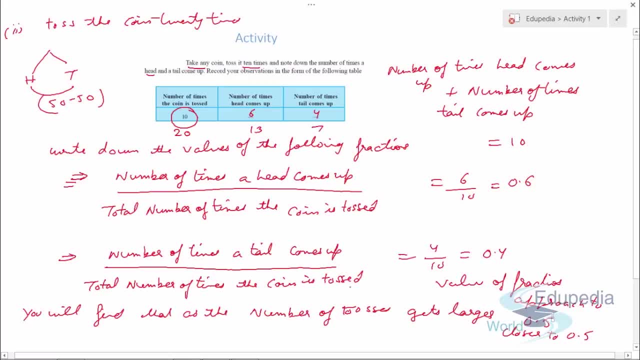 have a large data set, then the values of fraction will approach to 0.5. means that our values are neutral. So this is how we can approve our probability concept through the experimental approach by using this. So this is how we can approve our probability concept through the. 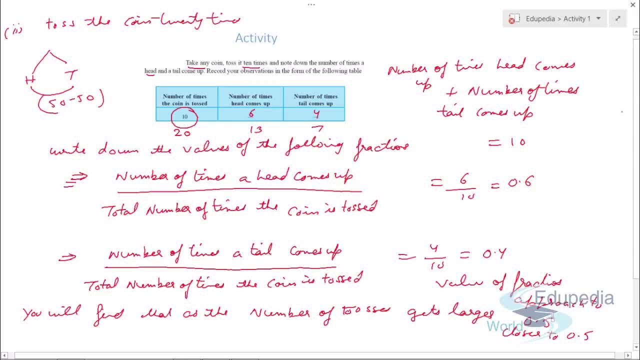 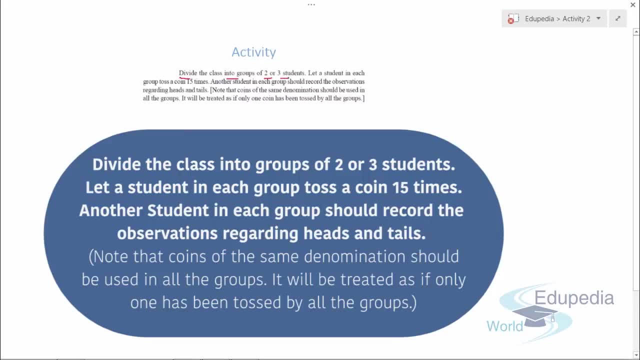 experimental approach by. So lets move on to our next activity, which is activity number two. this activity says that divide the class into groups of two or three students. right, Let's each student group toss a coin 15 times. another student in each group should record the observation. 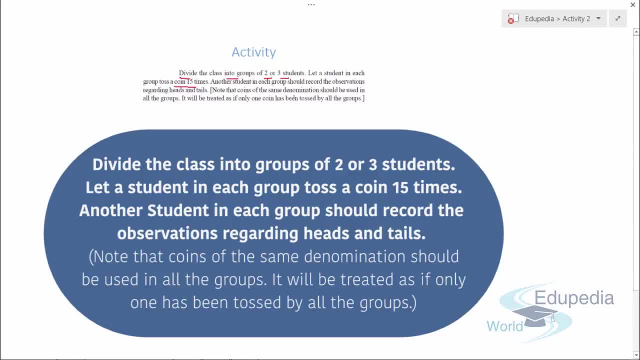 regarding head and tails, then note that coins of the same denomination should be used in all the groups. So the coins should be same and it will be treated as if they are only held Now one coin right. so the denomination should be the same right. so this means 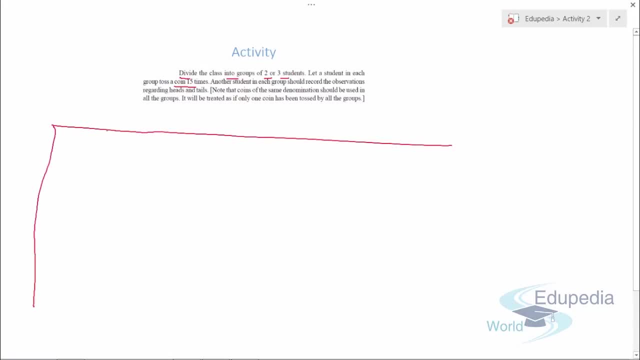 first we have to make a table like this. the first it comes out to be group, then comes out to be number of heads. right then comes out to be number of tails, right then comes out to be: we can say number of heads upon total number of trials, or we can say total number of. 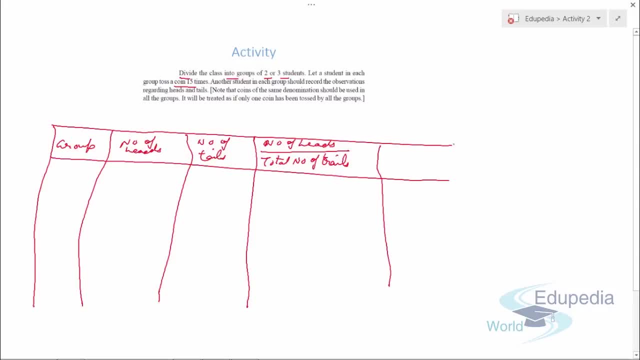 events, right? then comes out to be number of tails upon total number of trials, right? so let's say, for the group 1, the number of head comes out to be, let's say, 3. then number of tails comes out to be 12, right? So this will come out to be number of heads upon number of trials. 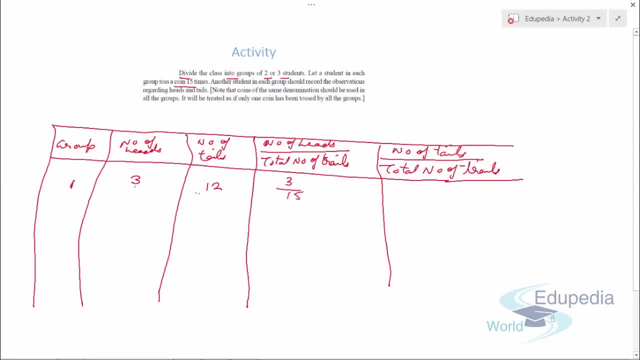 So it will be 3 upon 15, because it is 3 plus 12, right? Then number of tails will come out to be 12 upon 15.. So this is the first group, right? Let us say the second group again tosses the coin. 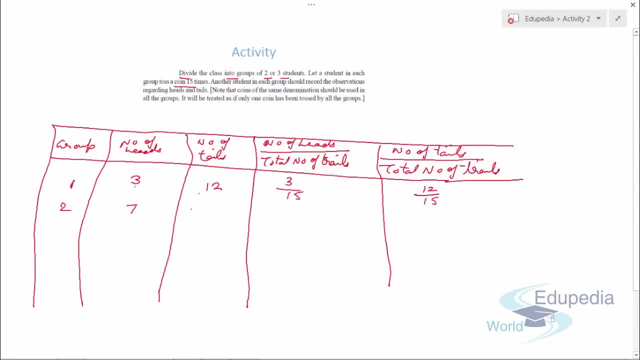 Then let us say, the number of heads comes out to be 7 times, number of tails come out to be 8 times. So this will become 7 plus 3 upon 15 plus 15.. So this will come out to be 10 upon 30, right. 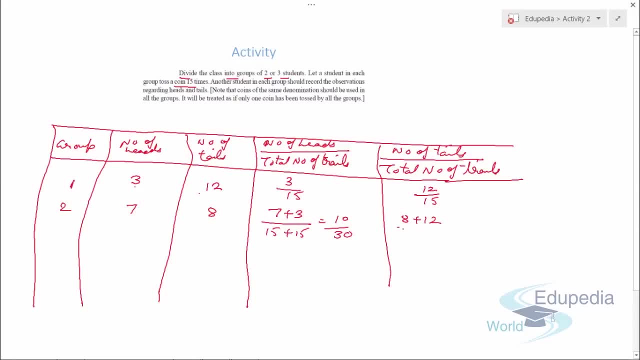 So, similarly, it will come out to be 8 plus 12 upon 15 plus 15.. So, which will come out to be 20 upon 30, right? So let us consider the next group, which is third. Now, the number of heads comes out to be 7 again, and number of tails comes out to be 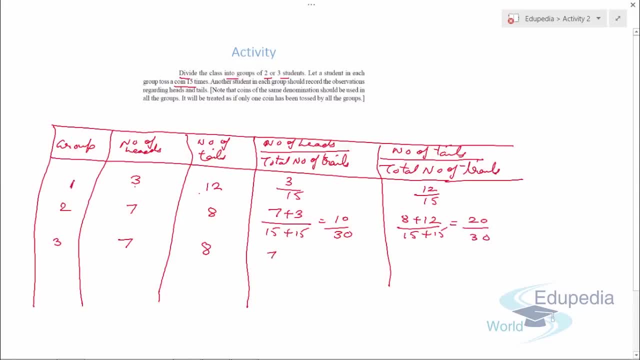 8, right, So this will come out to be now 7 plus 10 upon 15.. So this will come out to be 8 plus 10 upon 15 plus 30, right, So this will come out to be 17 by 45.. 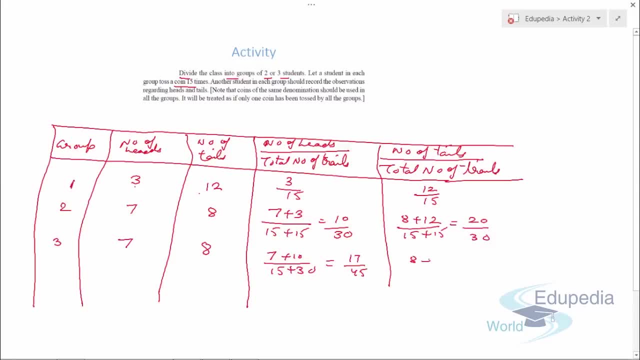 So this will come out to be 8 plus 20 upon 15 plus 30. So this will come out to be 28 by 45, right? So what you can observe over here is so, as we are increasing the number of toss, let. 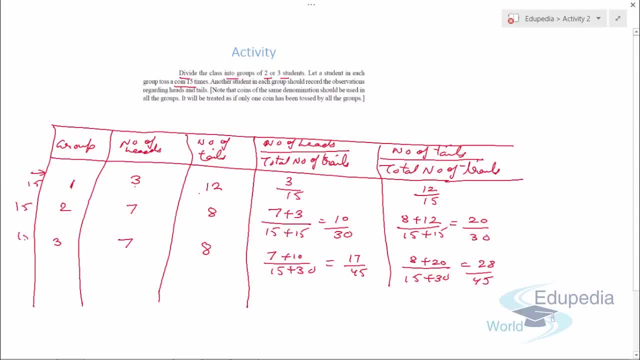 us say 15 over here, 15 over here, 15 over here. So we can say that the value of head and tail is again approaching closer to 0.5, right? So this means to approve our experimental approach to, or we can say to get a better. 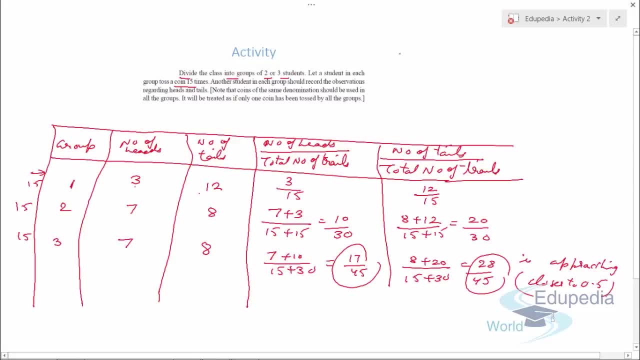 estimation of the probability or likely happening of event. we need to have a lot of data right. So we need to have a sufficient data so that we have a neutral kind of our experimental approach. So this is how we can use the activities to prove the concept. 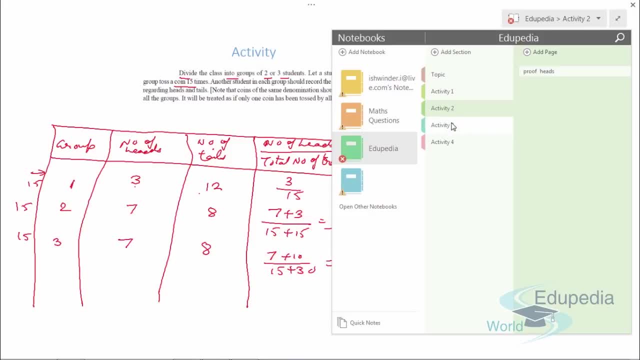 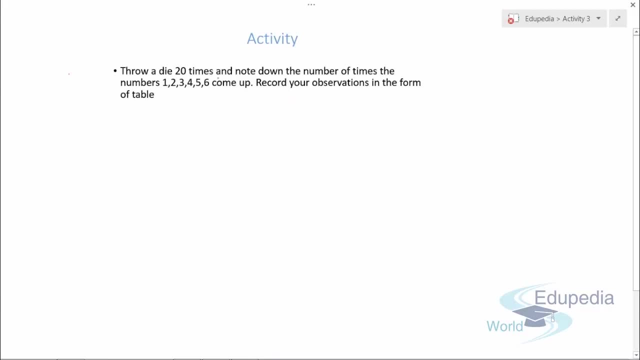 So let us move on to the next activity, which is activity number 3.. Now activity says that throw a die 20 times and note down the number of times, the numbers 1,, 2,, 3,, 4,, 5,, 6, comma, and you need to record your observation in the form of table right. 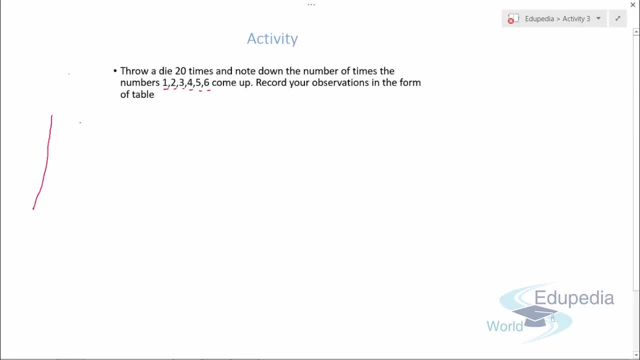 So first of all, draw a table right. You can say number of Times a die is thrown right, Then over here, number of times These scores turn up right. So let us say, over here we write 1,, 2,, 3,, 4,, 5,, over here we write 6.. 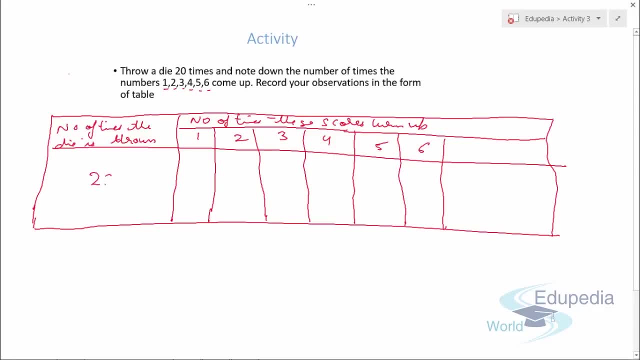 Let us say we have thrown a die 20 times, So we write 20 over here. This comes out to be 5 times. Let us say: this comes out be 7 times. right, this comes out to be, let's say, 3. comes out to be 4 times. so let's say this comes: 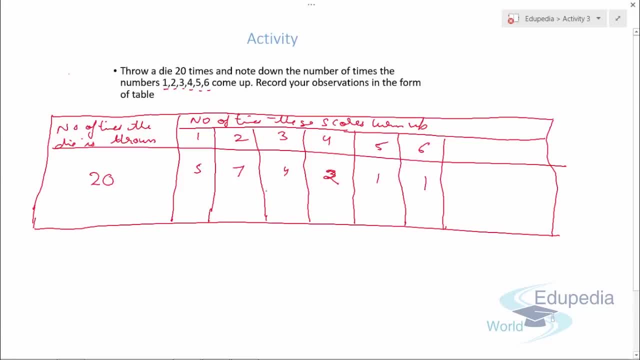 out to be 2 times, that this comes out to be 1 1 time. so we need to check. the sum should be 20, right? so it is 5 plus 7, which is 12. 12 plus 4 is, which is 16. 16 plus 2 is 18. 18 plus 1 is 19- 19. 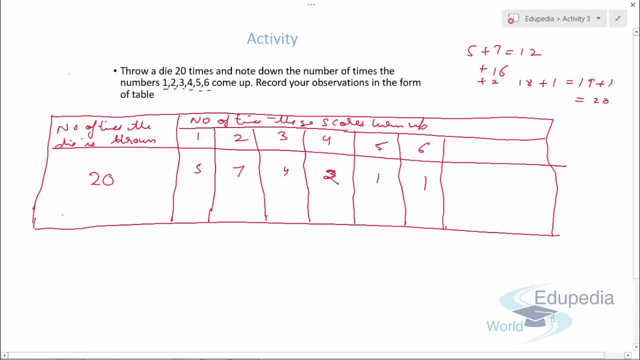 plus 1 is 20, right? so these are all the observation. now let's say number of times 1 turn up, right? so this will come out to be this part divided by this part, so which is 5 by 20. similarly, we can say number of times 2 turn up, so which we can find 7 by 20. similarly, we can say: 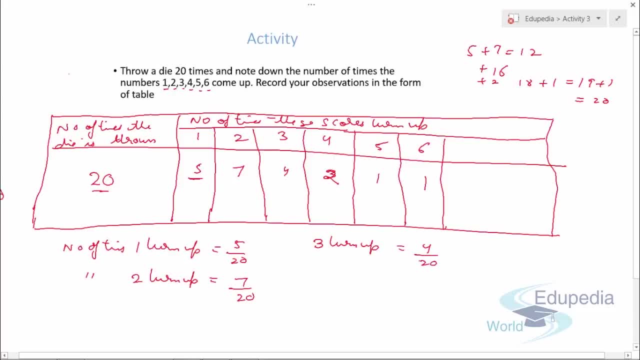 the number of times 3 turn up, 4 by 20. then, similarly, we say that number of time the 4 turns up, 2 by 20. again, how many times the 5 turns up. so which is 1 by 20. so which is 1 by 20, right. 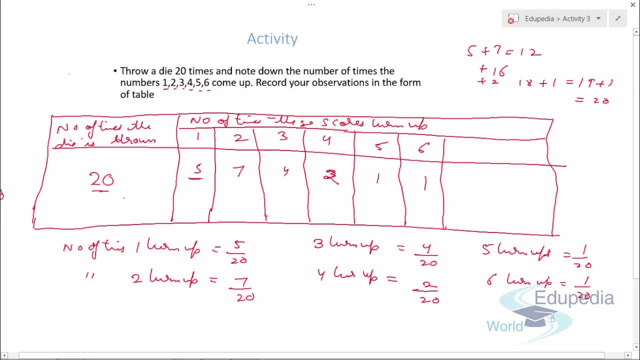 so this is all the probability when the die is thrown, 20 times numbers turning up right. so let's say, if we increase the number from 20 to 30, again we will have a different observations. so then for 40 we'll have another different observation. so what we can observe is that 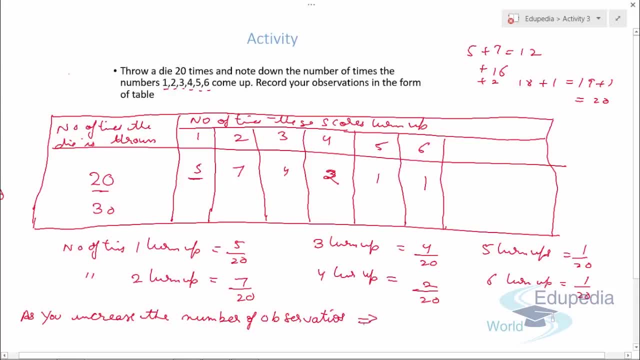 as you increase the number of observations, what you can observe is that, where 4, 1 of each fraction will approach to 1 upon 6, right. so again, this approves our experimental approach that through activities we can approve the concept of probability, right. so let's move on to the next activity, which is activity. 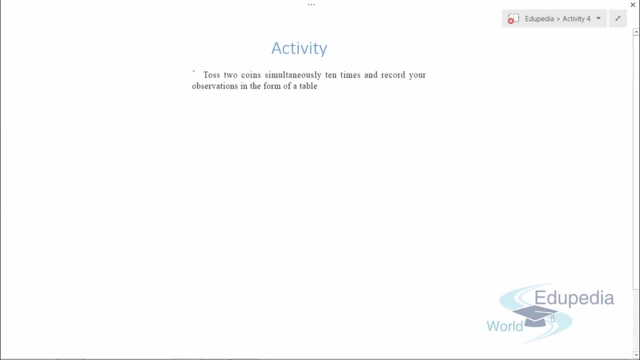 number 4 on, which is also a last activity for this video. this activity says that toss two coins simultaneously 10 times and record your observations in the form of table. so first of all draw a table number of times the two coins are tossed, right, then over here we can say that. 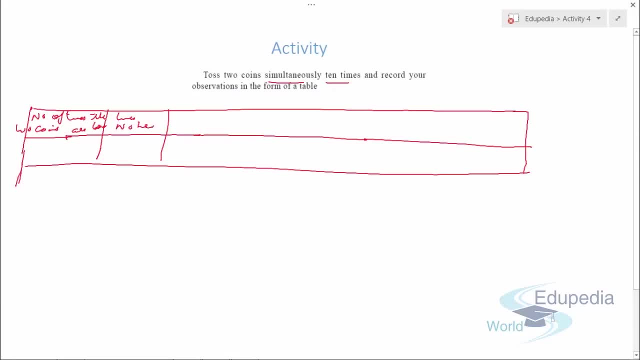 number of times. no head comes up. right over here we can write one. head comes up, over here we can write two head comes up, so let's say the coin is tossed right. so let's say the coin is tossed right. so let's say the coin is tossed. 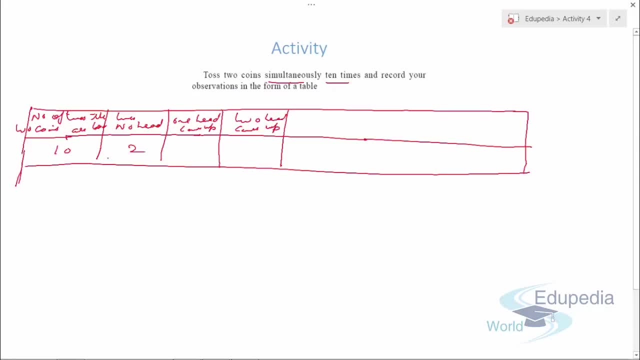 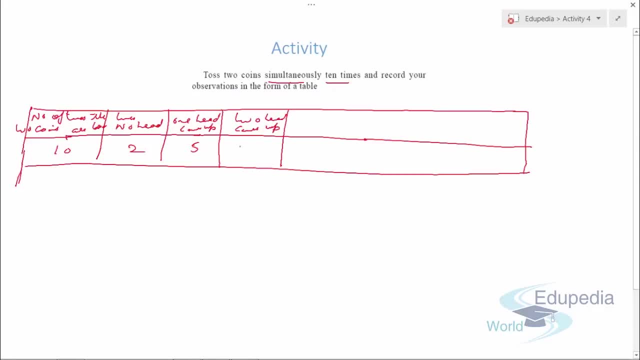 let's say five times and two head comes out to be, let's say, three times. this is the probability now. so what you will observe is: let's say we find the value of fractions, so let's say value for no head. it will be 2 by 10 and 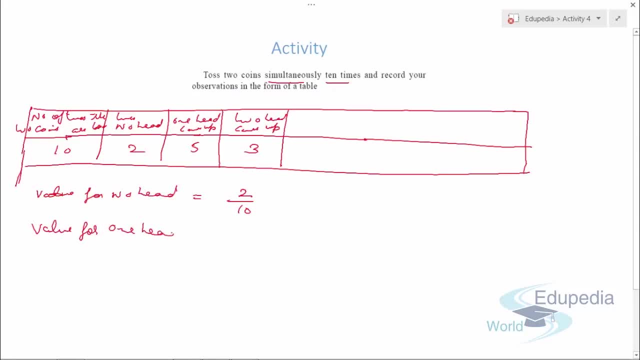 value for one head coming up is 5 by 10 and value for two head coming simultaneously is 3 by 10 right now. so this is all the probability of coming: no head, one head and two head simultaneous right now. again, if you increase the number of 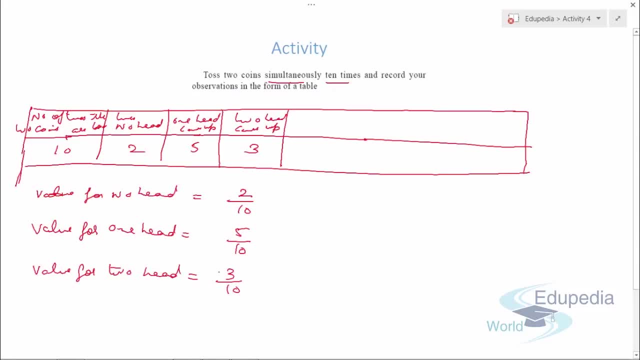 observations, then the value of probability will change, right. so what you will observe is: so, as you increase the value of number of observation, this value will approach. so this value will approach to 0.25, right, and this value will approach to 0.5, and this value will approach to. 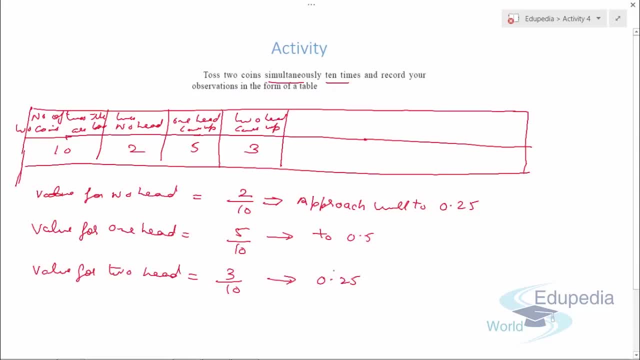 0.25. so this again approves that we can apply the activities through experimental approach to approve our concepts of probability right now. these are all the activities we have discussed so far for the probabilities now, what is a general formula? or we can say what is a general definition? 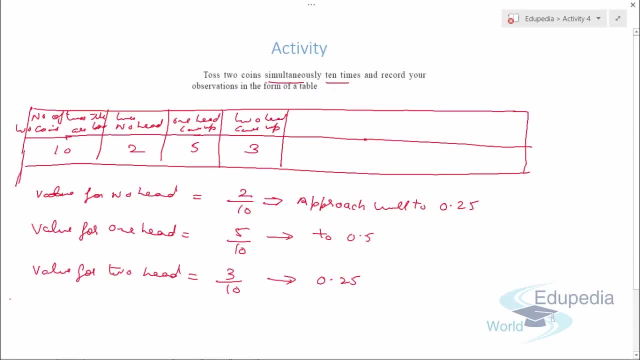 for the probability, right, so you have to note this point very carefully right now. so you have to note this point very carefully. right, so you have to note this point. right, so you have to note this point very carefully. right, so you have to note this point very carefully. 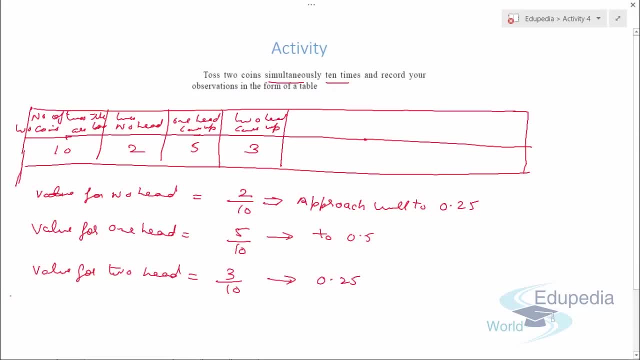 because for this definition only you will solve whole chapter related to the probability right. so the definition says that let n, we can say that let n be the total number of trials right and we can say that the empirical probability, empirical means equal, likely, which is denoted by p e. so the symbol p e refers to 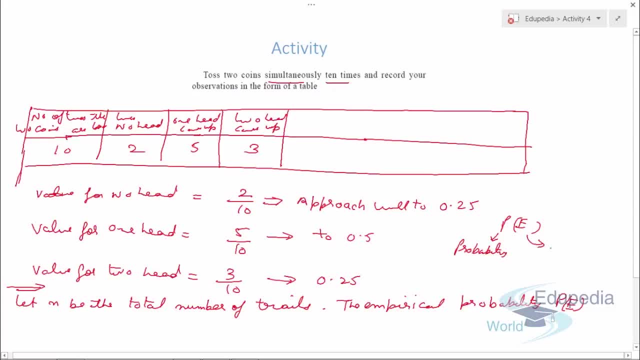 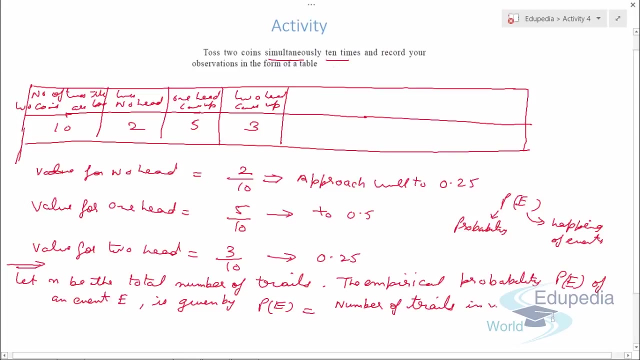 p means probability and e means happening of events. right, so this is a representation of an symbol. so p e of an event, e is given by. we can say p e equals to number of trials in which event happened upon, total number of trials. so this is the definition and the formula for solving any kind of probability.